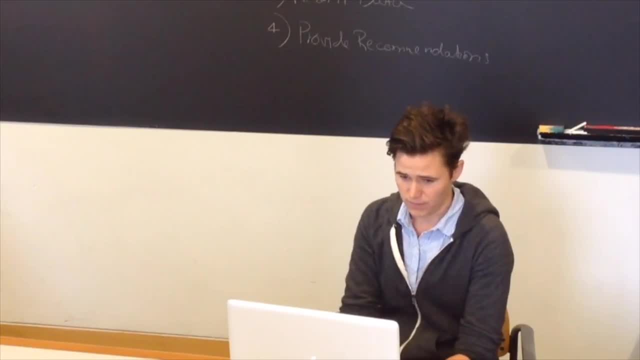 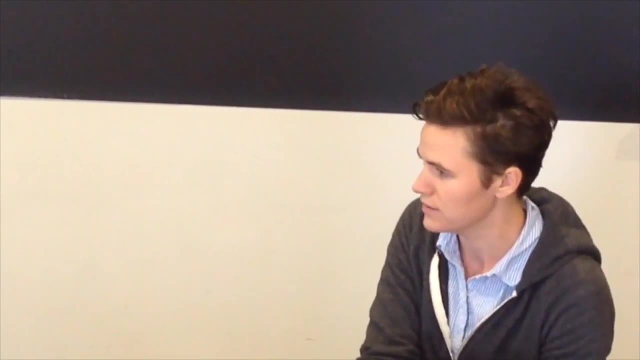 so far it's been effective. From the point of view of scientists and environmental advocates, it's a success. Pollution has been vastly reduced since implementation of these policies, and this is a tremendous achievement. So why stop now? That is our argument. There are 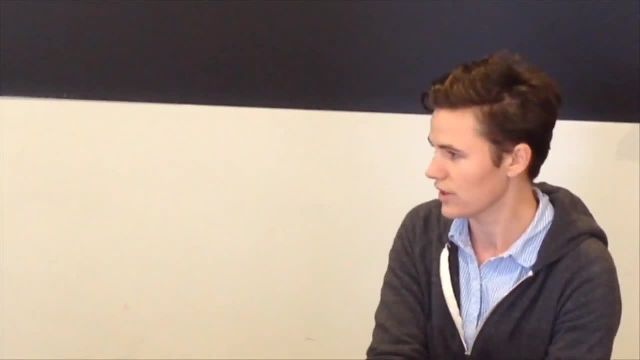 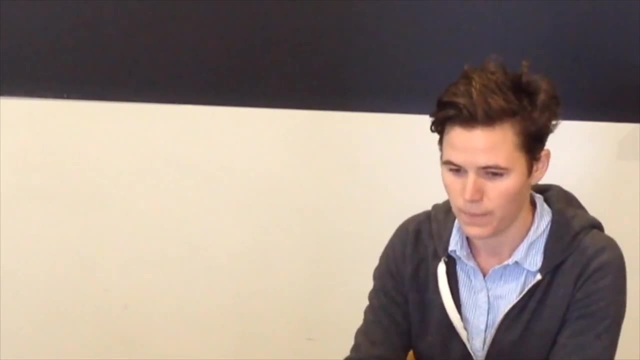 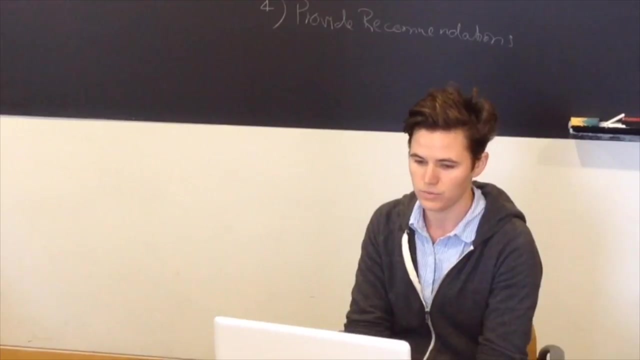 still extremely endangered ecosystems in this country, and industries are constantly inventing new products that could have new negative effects on the environment that we're not yet aware of. So the study we conduct to challenge the Heritage Society's claims will have four parts. First, we'll focus on science-based policy. We'll focus on the protection of natural. 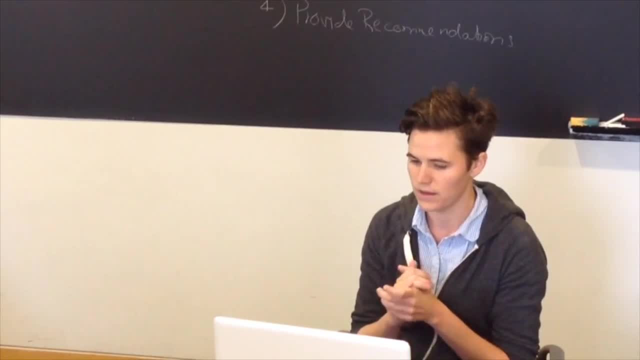 benchmarks. We'll also focus on public opinion. We'll propose an administrative review of the EPA and a review by the Justice Department. So for our first pillar, the scientific measurements, we'll hire an outside team of environmental scientists to evaluate air and water quality. 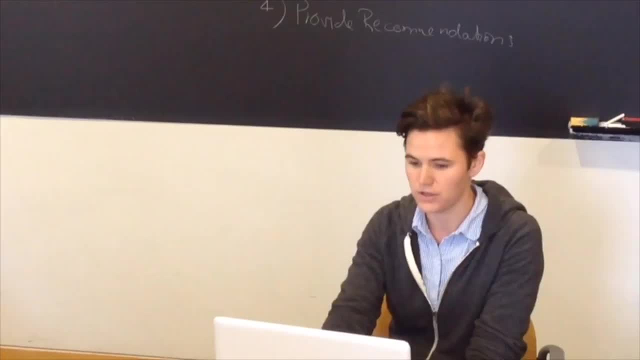 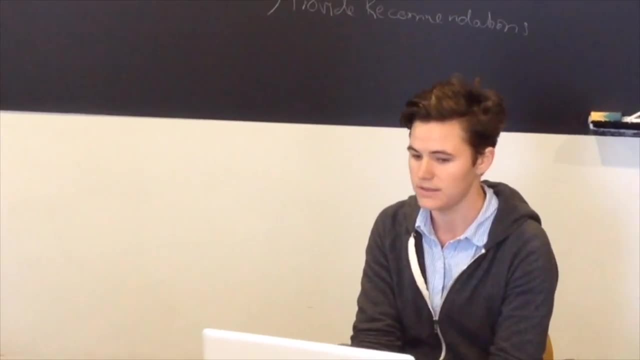 and how it has improved since 1970.. Scientists must also prove that threats to the health of our environment, to our clean air and water, still exist and that regulation of anything should be expanded and improved, and not reduced or terminated. We need to frame our study to focus. 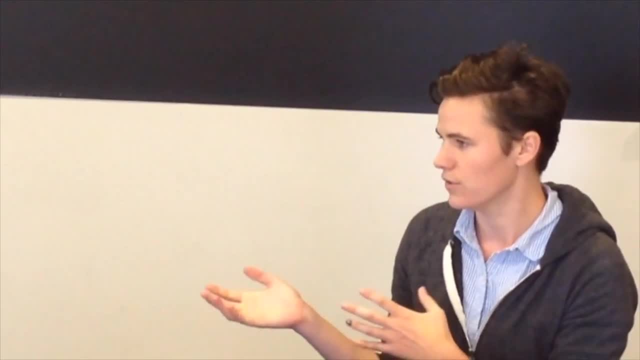 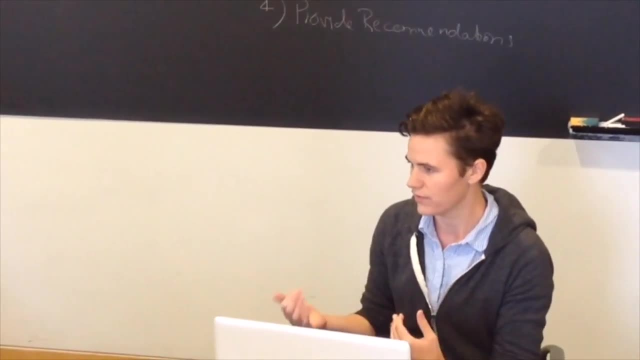 on scientific results to counter the Heritage Society's focus on economic results. We will design a study based on science and numbers, because that is how you will measure the efficacy of a program like the Clean Air Act. So focus on how you improve vehicle emissions, how fish and 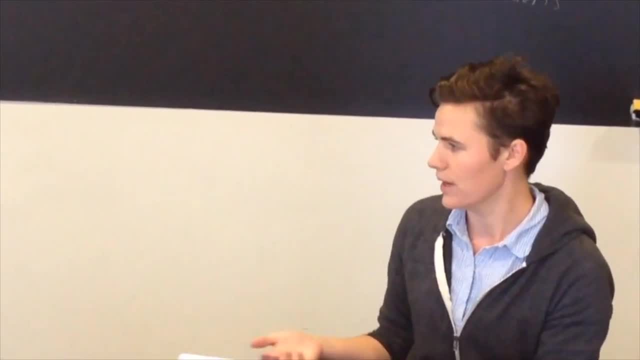 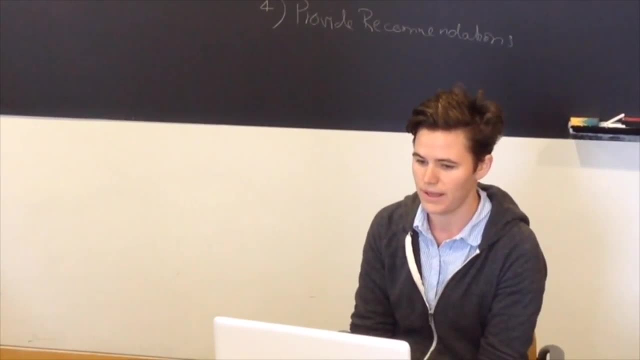 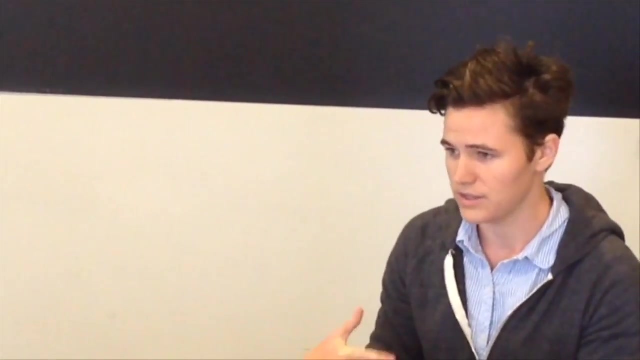 bird populations have bounced back, and this will help legitimate our study in the eyes of the scientific community. We can also come at this from an angle that will satisfy the business community and Congress. We can require companies to maintain certain air quality standards as a means to spur innovation. 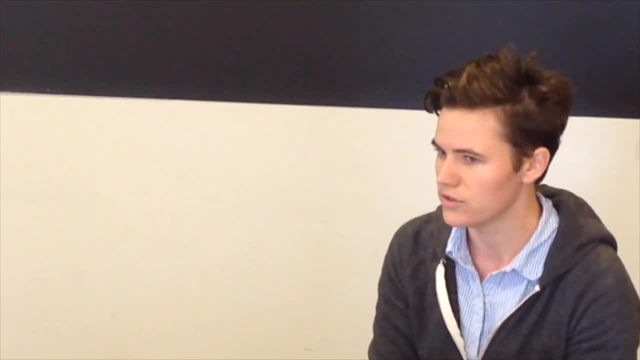 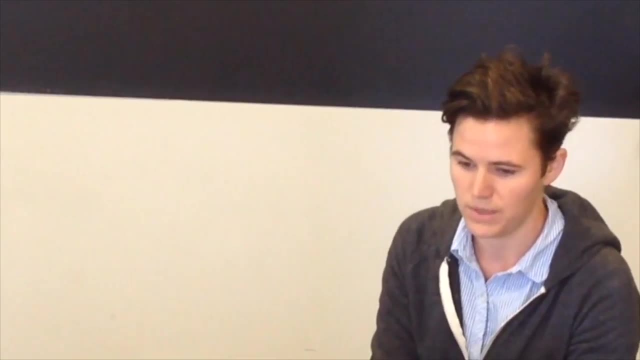 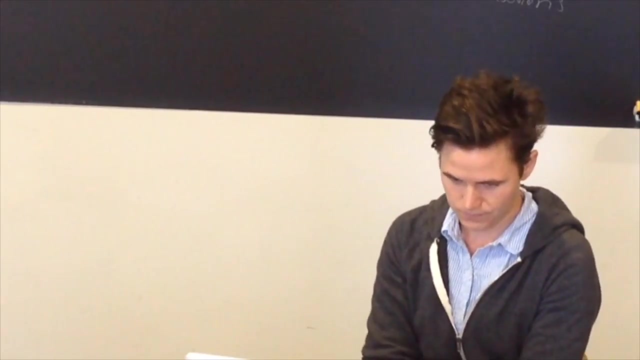 We've been innovative in this regard so far. We've invented cleaner fuels, renewable energy, and we believe that the American people can invent even better, cleaner technologies, and the regulation will help inspire that. Our second component: we'll focus on the public's stance on the issue of environmental protection. 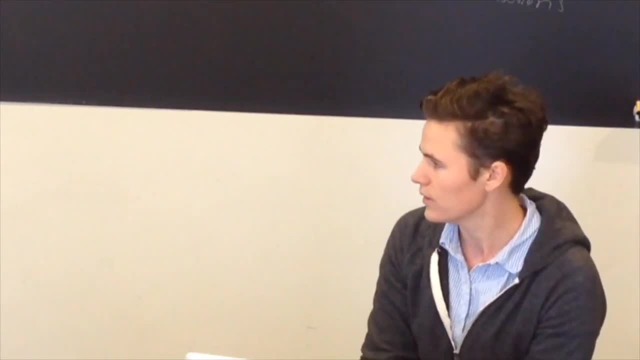 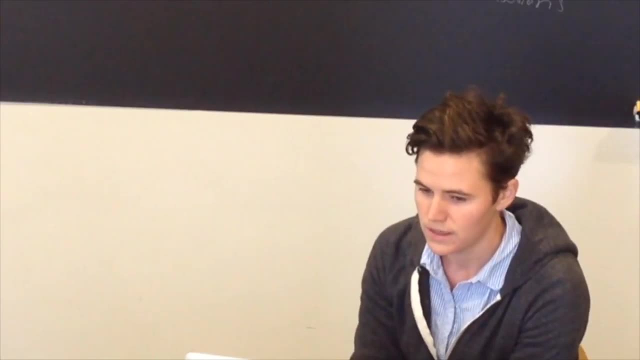 We're in an unprecedented era in environmental awareness, and the public is completely behind it. I'd like to bring your attention to a very revealing ruling that just came out. in the last few weeks In Massachusetts, two men used their lobster boat to block a coal shipment from passing through the channel. 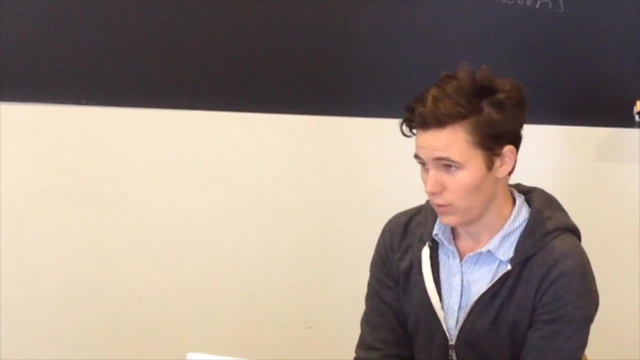 on its way to Brayton Point Power Plant. The men were on trial for several counts and faced several years in jail, and the judge ruled that he approved the use of natural gas. The judge ruled that he approved the use of natural gas. The judge ruled that he approved the use of natural gas. 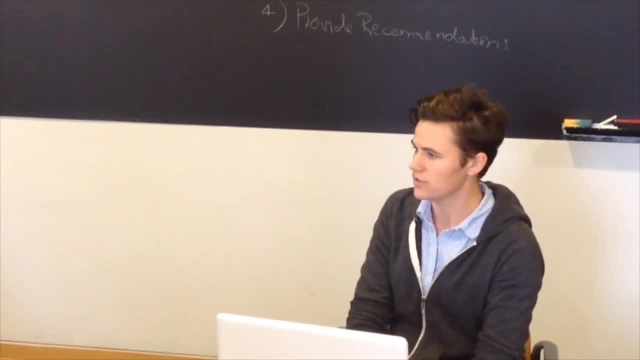 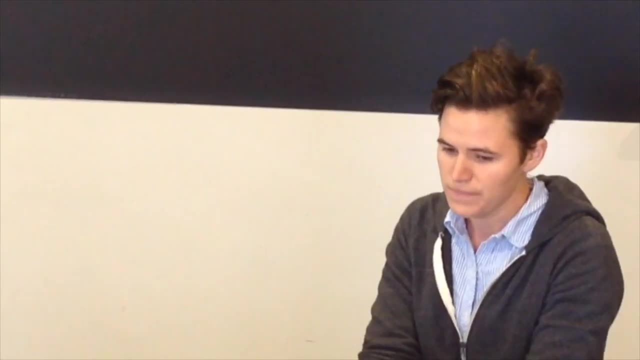 They approved the use of necessity as a defense for their actions. In order to use the necessity of your friends, you have to prove that you are in clear and imminent danger. In this instance, the defense argues that the men in their communities were in clear and imminent danger of climate change. 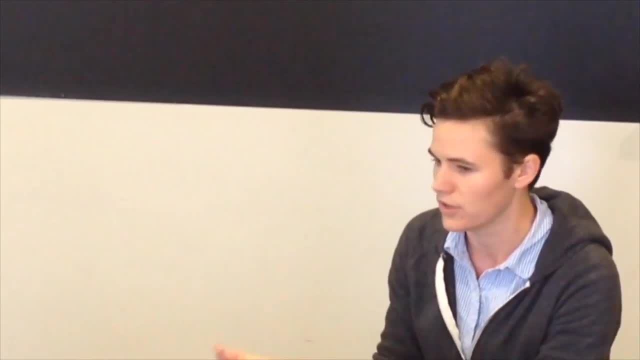 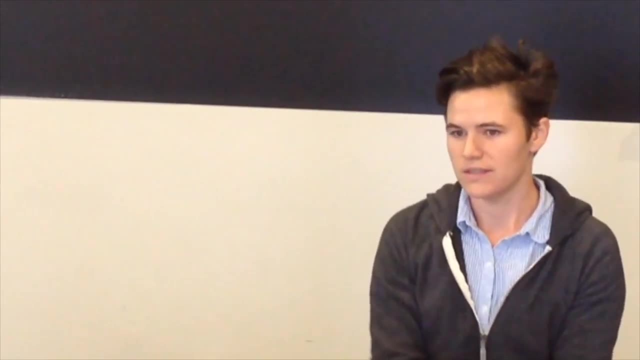 The judge decreed they had no legal alternative to protect themselves and their communities other than to try to block the coal shipment. The prosecutors subsequently dropped the charges. Obviously, this is a totally unprecedented case case. This is an exciting time for environmental progressives. Judges are 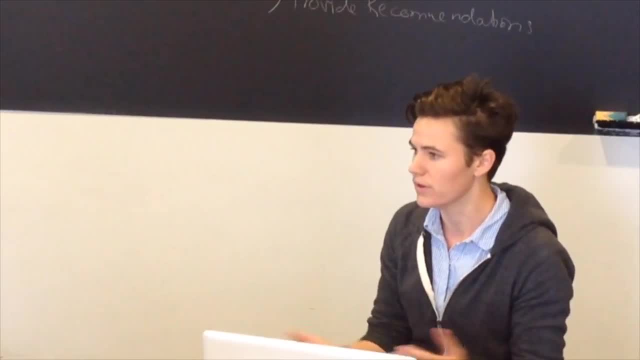 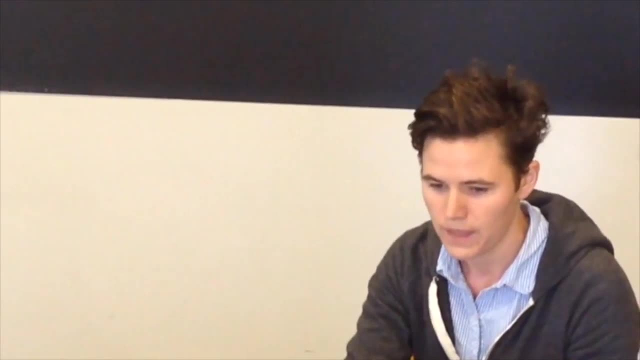 going rogue on this issue and are allowing people a lot of rooms to maneuver to fight environmental problems. So we want to design a policy review that involves the public energy as much as possible. So we're going to educate the public. We're going to use some of our funding to organize conferences and 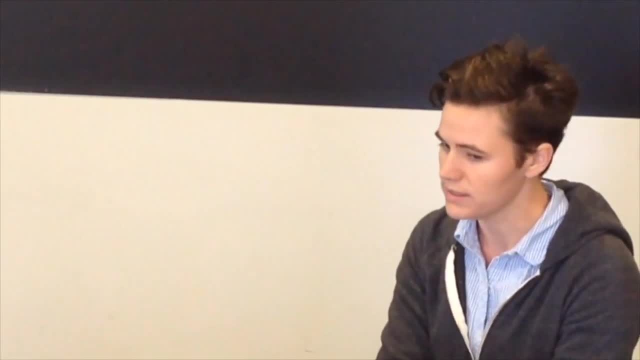 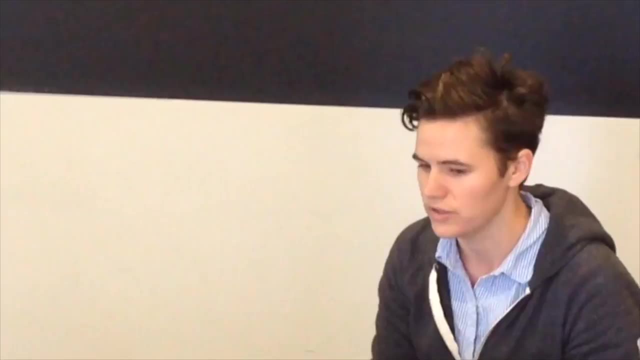 smaller community advisory committees. These committees will call small meetings in their communities and discuss the EPA's community control policies, and they can weigh in on whether or not they think those policies should continue at this time. This method will give our study legitimacy in the 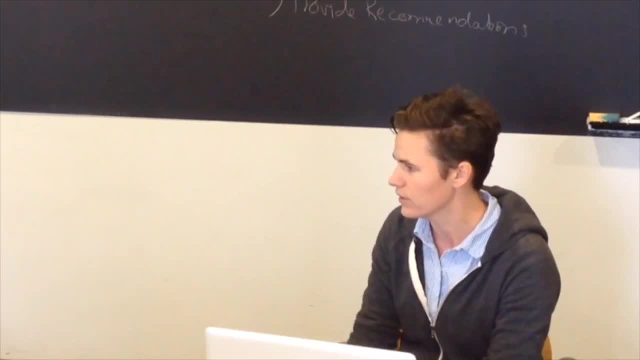 eyes of the public and in the eyes of Congress, who depend on the public for voting. I highly doubt the Heritage Society did a public assessment or reached out to the public in their view, so this will give our study that added legitimacy that we involve the public opinion And then, come election time, the public will play a.